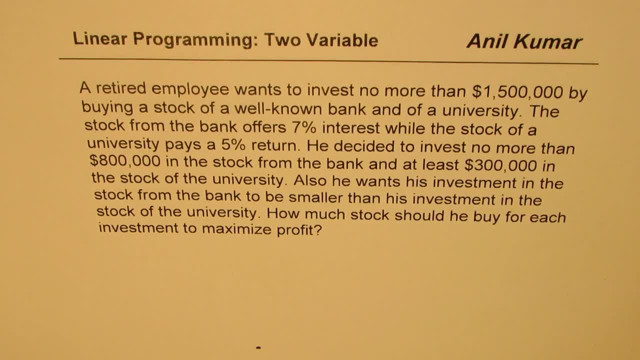 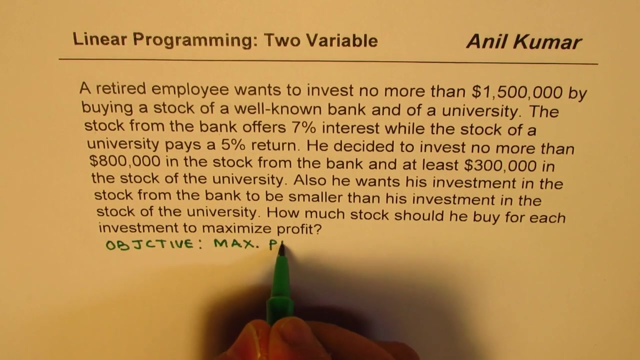 and then look into my suggestions. Now, whenever we begin with solving linear programming questions, we should keep in mind what is required. What is required is to say what is the objective Now, in this case, the objective is to maximize profit. So objective is to maximize profit. How can we maximize profit? That is what the 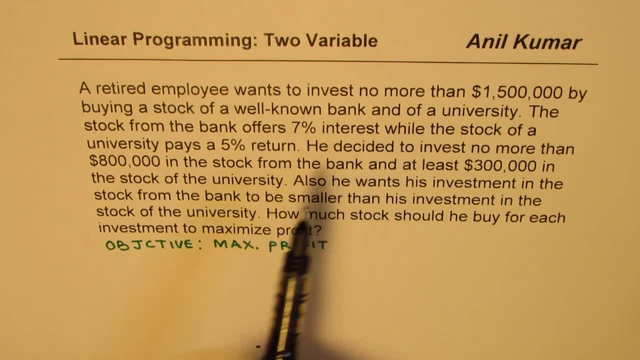 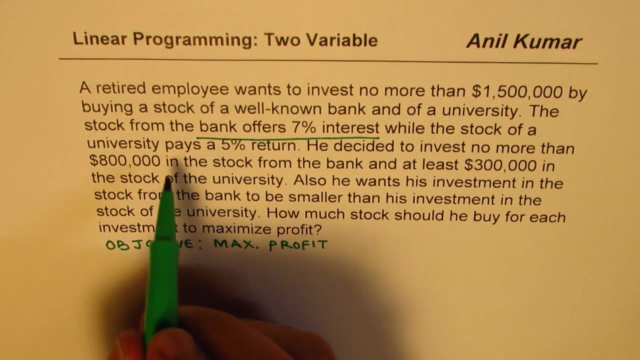 objective is. We are looking for investments in two places. One of them is the bank, the other one is the university. now, bank offers 7% interest and the university pays 5%. okay, so let us assume that out of the total amount, B is invested on. 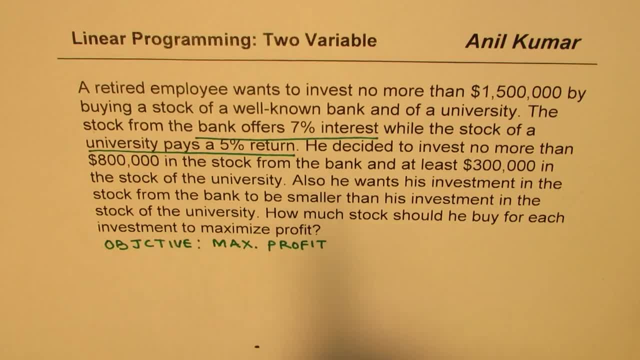 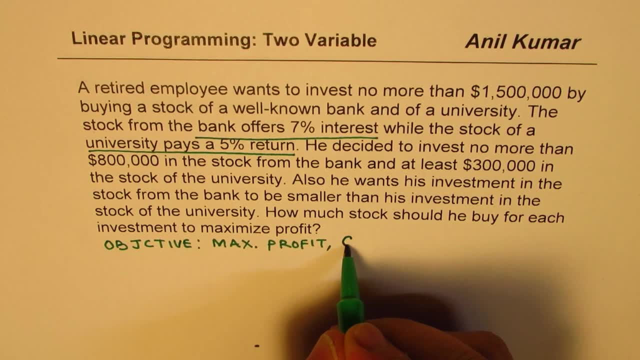 bank and U is invested on university right, so so the maximum profit, which is definitely in dollars, so it's a cost- let's say P, okay, earnings or okay, let's say profit- is equal to 7% from the bank. so 7% means zero, point, zero, seven. 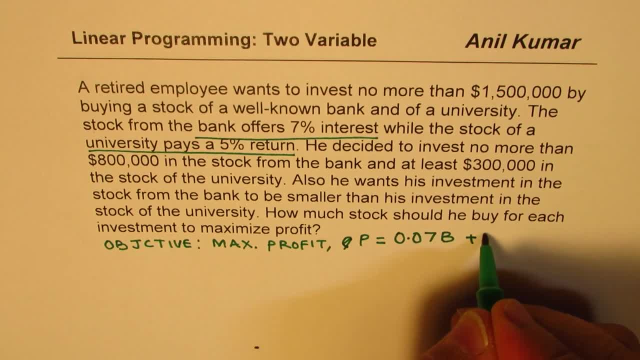 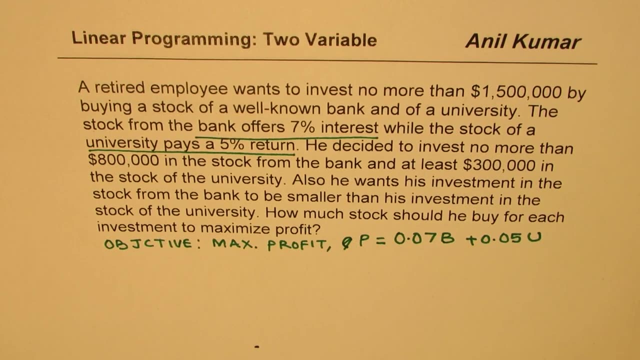 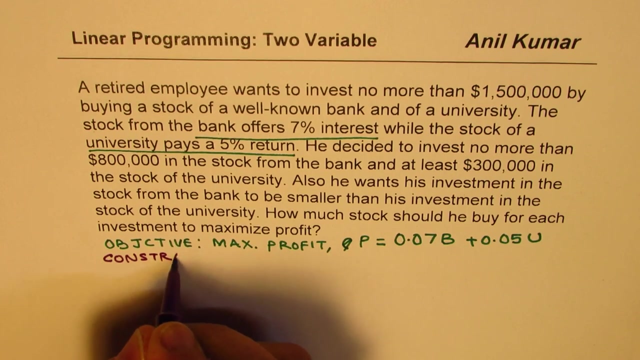 okay on whatever is invested in bank, plus zero point zero five on what is universe invested in the universe. so that becomes the objective. now to find the solution. what we could do is we could first write our constraints okay, plot those constraints, find the corners and then figure out which point gives us the maximum profit. so these are the steps. 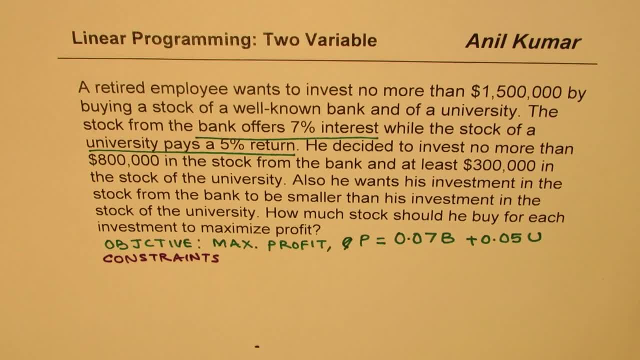 involved right now. amongst the constraints, to begin with, we know that the total amount P- I'm total amount B plus U is 1500, right. so the first constraint here is that we have an amount which is 15,000 right. so we'll work in. 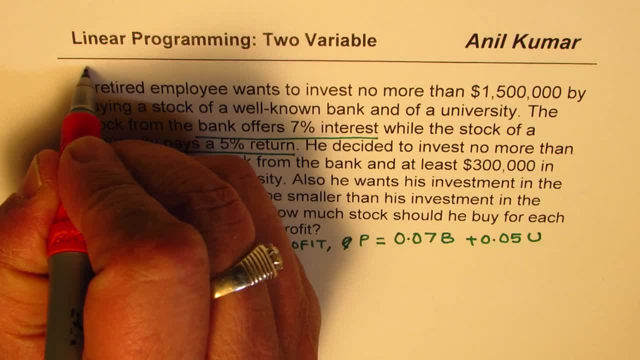 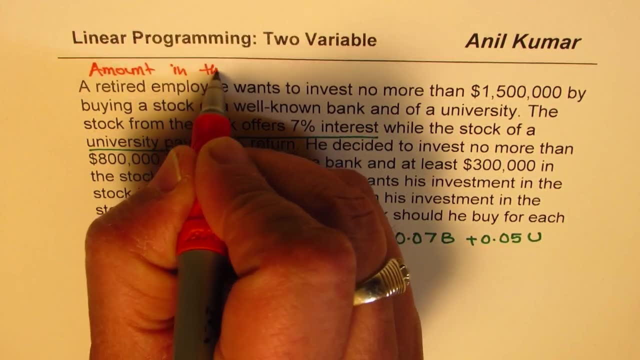 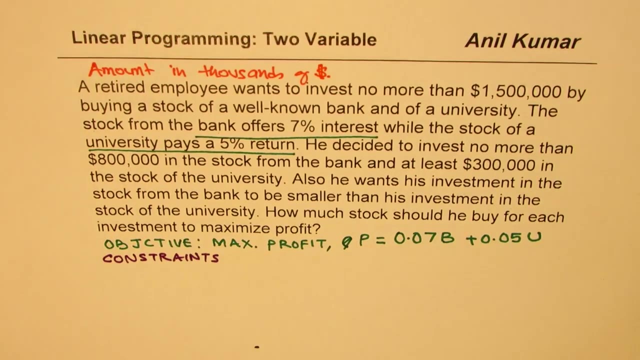 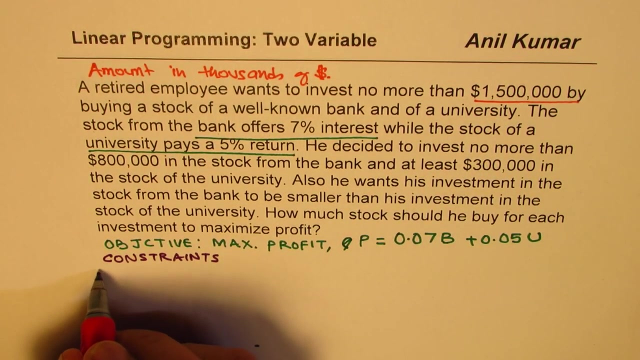 thousands of dollars. let's work in thousands of dollars, so we'll work in amount in thousands of dollars. okay, I will actually solve the P the question here in this page and therefore I'm trying to economize on the space here. okay, so total amount is: So, since we are working in thousands of dollars, let's say this amount here is bank plus university. 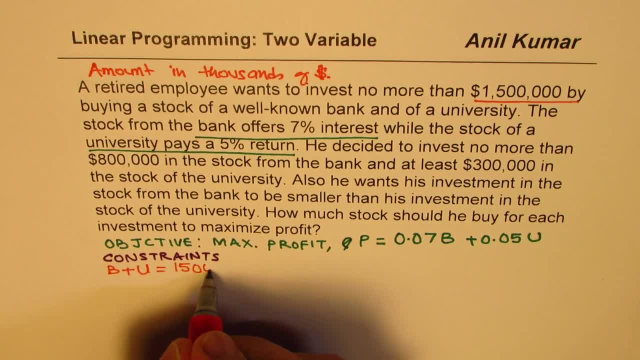 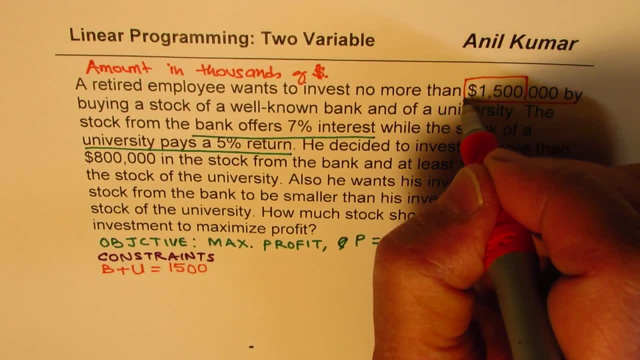 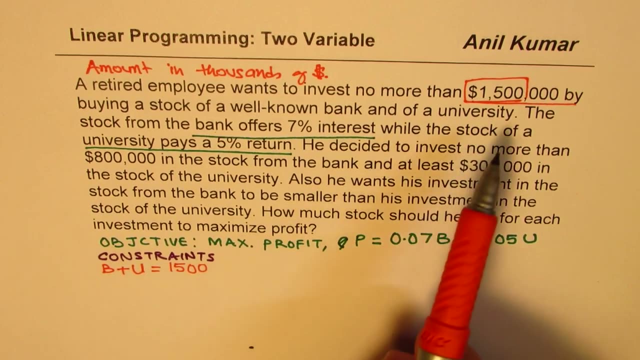 is equal to 1500, right, We'll write in hundreds. We know all these amounts are in thousands of dollars. okay, So we are only writing in thousands. Now he decides to invest no more than $800 in the stock from bank. 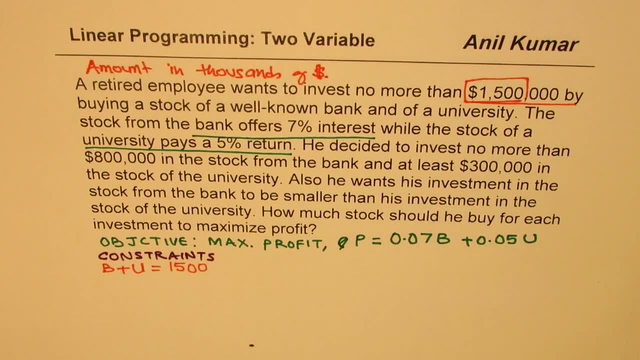 So that is another constraint. So we'll use different things so that it becomes simpler for us to graph. So: no more than $800 in stock from the bank. Okay, That means bank B is less than equal to 800,000,. we'll write 800, correct, fine? 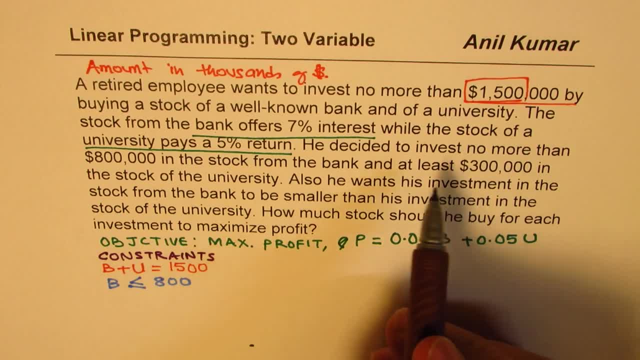 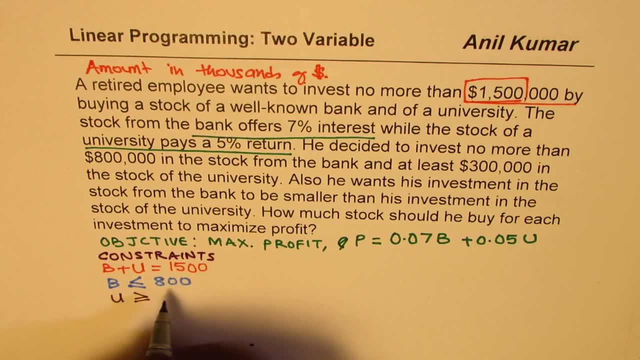 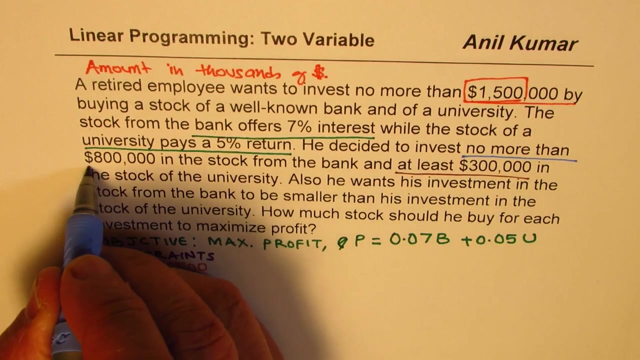 And at least at least $300 in the university. So university has to be greater than equal to 300. So at least means greater than equal to right. Okay, And we have also taken care of no more than 800 for bank, okay. 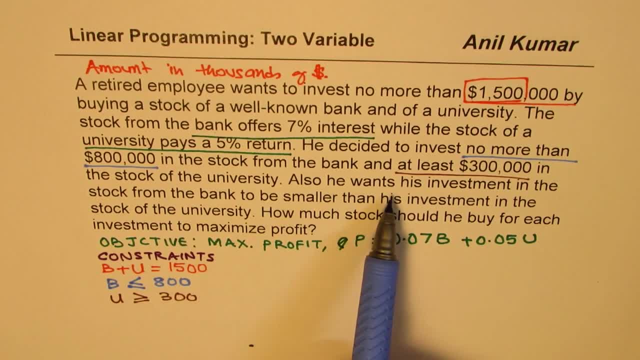 Also, he wants his investment in the stock from the bank to be smaller than his investment in the stock of the university. So that is another constraint, That is, He wants the investment in the stock from the bank to be smaller. So so the bank is less than university, correct? 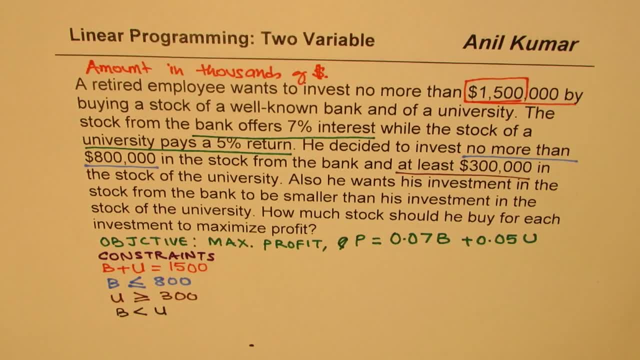 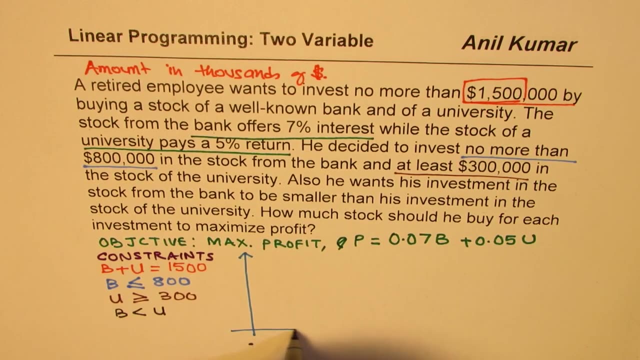 So these are all the constraints which we have to work with. So, based on these constraints, let's sketch our graph. Let's do it here. Okay, Okay, So let's do it here. So, always, we are working in quadrant one, since everything is positive, right? 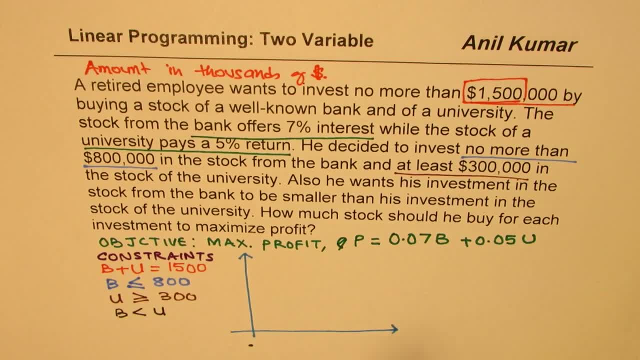 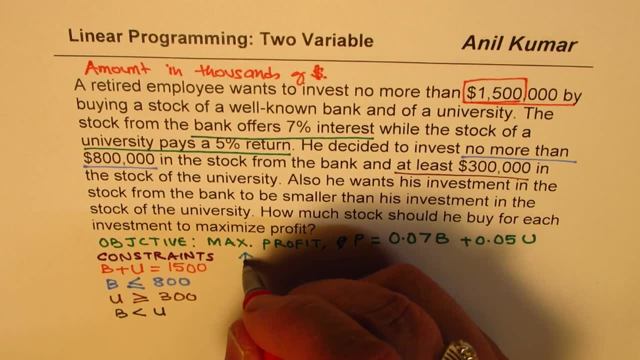 So the very first graph, which is the sum of money which we have is 1500, gives us two intercepts: 1500 for U, 1500 for B, right. So that gives you a diagonal here. So that sets up our boundary. 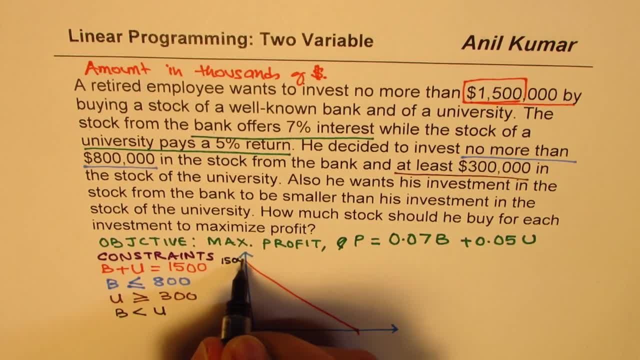 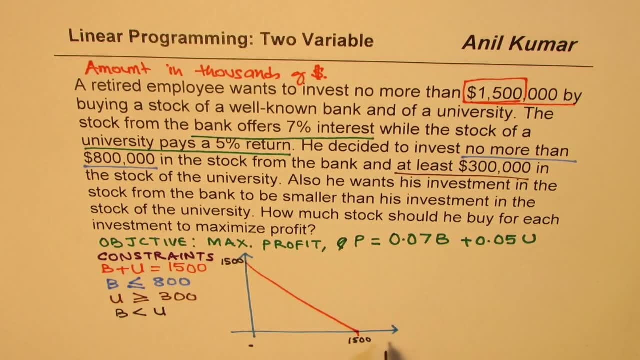 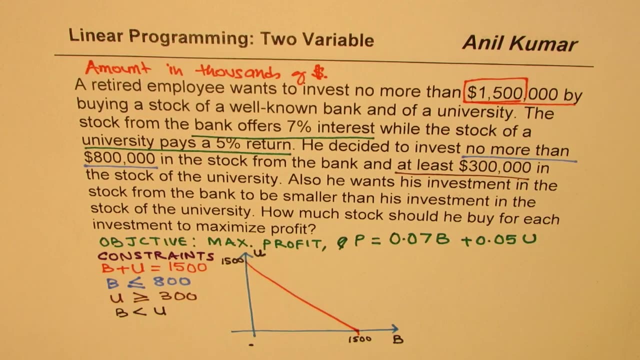 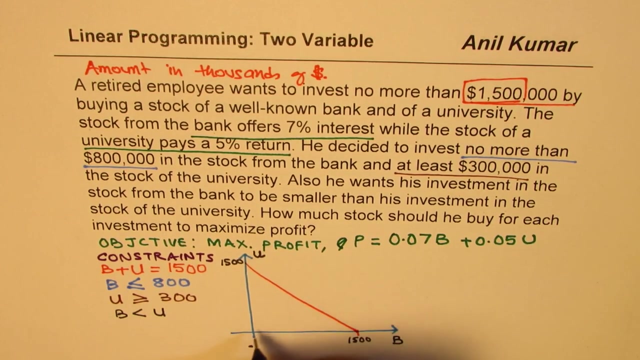 So we have 1500 here. So that sets up our boundary. all values are in thousands. right, We are taking bank on this side and university on this side. okay, Now we want bank to be less than equal to 800.. So let us say this is: 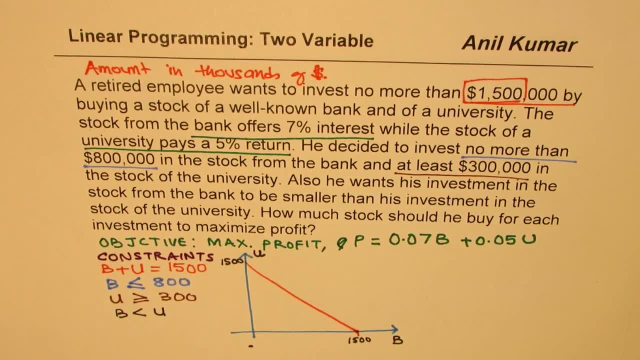 somewhere. here is the midpoint. We do have a graph for midpoint also. So let us say: 800 is here, right, So the color is blue. Let us say: this gives us 800, okay, So we are on the left side of this. 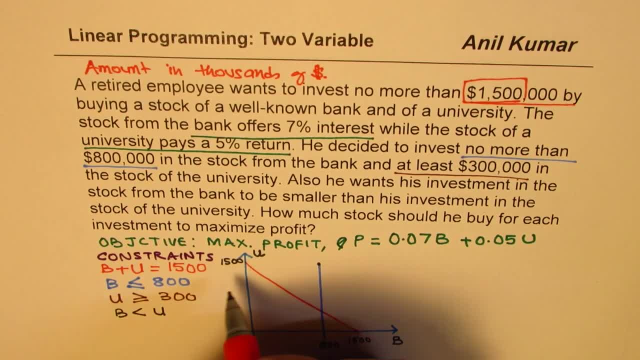 We are busy below the orange line right. So if you are sketching the graph it is kind of like this: right, Here we are on the left. So B is less than equals to 800.. So it is less than So. 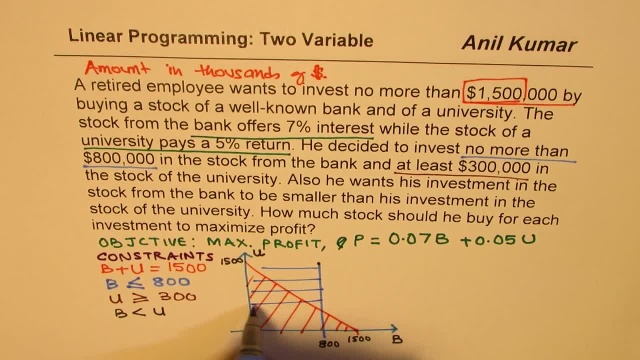 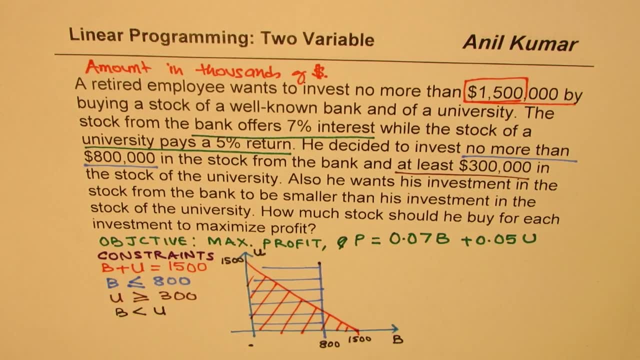 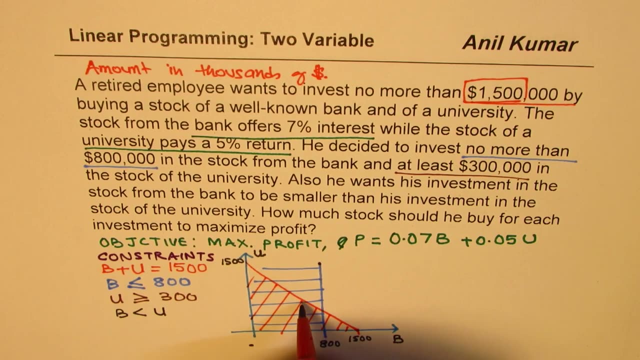 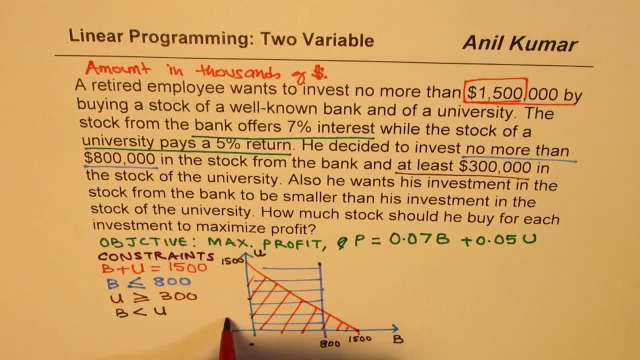 300 is somewhere here. okay, So we are having more than this. So that gives us a university. Now, the last one here is that the university is less than or equal to 300, rupees on a divider, correct? Now will junk be for salary? Well, that is entirely up to the question. 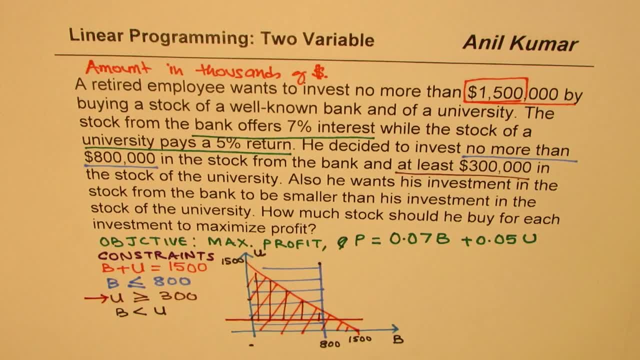 No cum laude. No, no, I think that 1.4 billion, Oh cool, The difference anywhere, which is very far, I am thinking on the bottom of the solution- Key三 triple is zero. I am not going to go into detail if you are not sure as to where exactly does it belong. 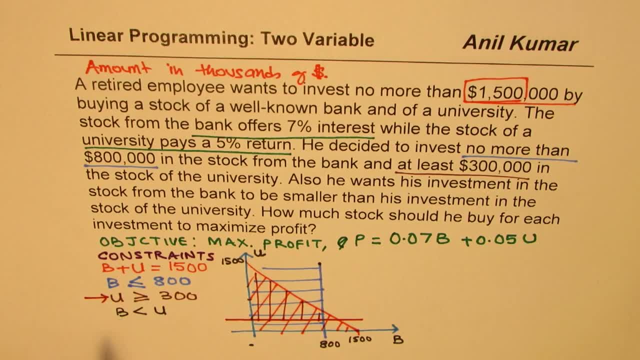 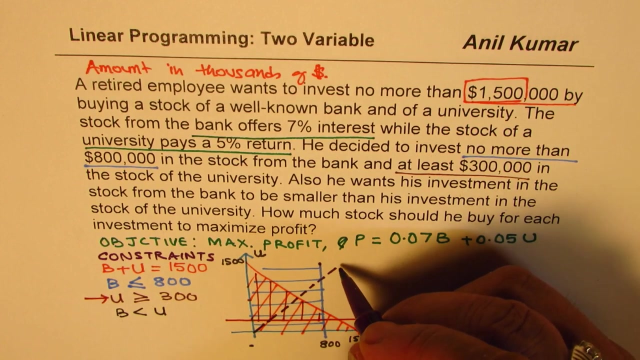 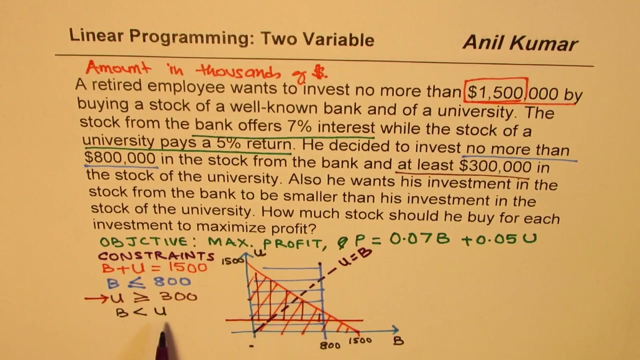 higher than b. so what we could actually do is they're not equal to right so. so university is this side. we could draw the line right going through the center with a dotted line. so this is the line which gives university equals to bank. but we need university to be higher, so 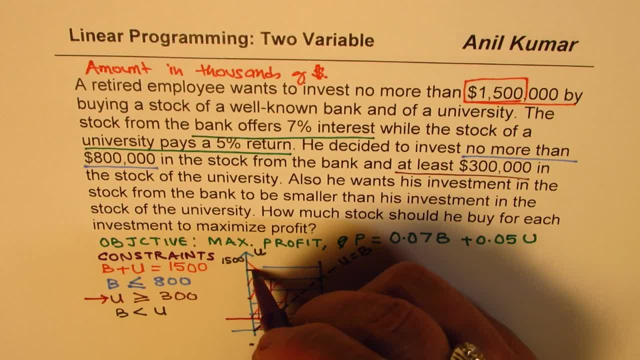 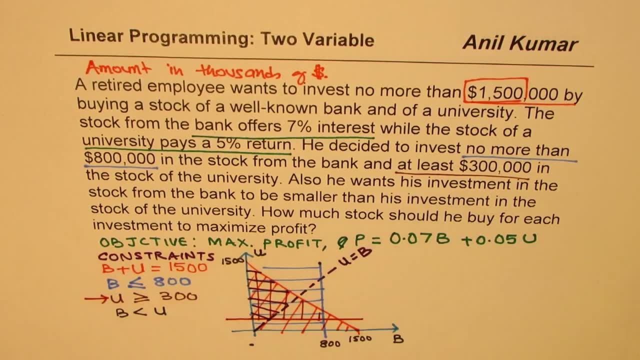 that gives us the area which we are really interested in. that is a sample space. do you see that? that is a sample space. so the points of interest on this sample space are going to be: one is 1,500, then we have a point here. we have a point here. we have this point also, right. 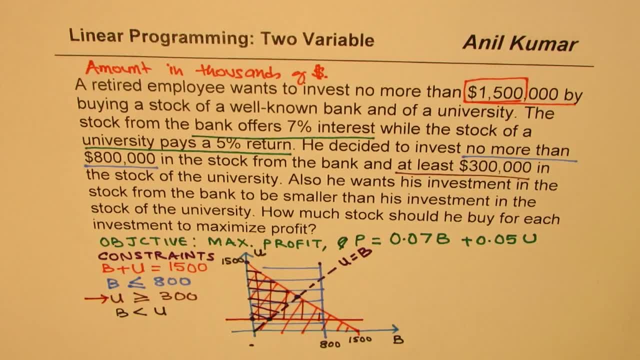 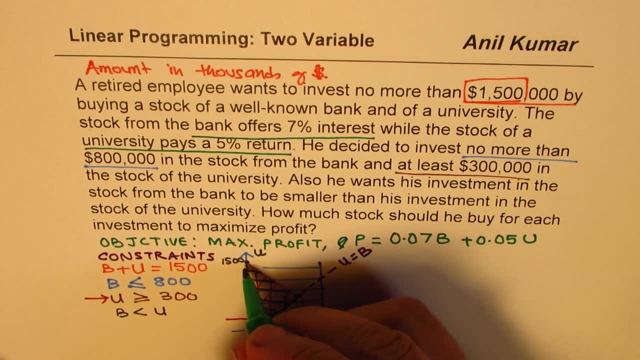 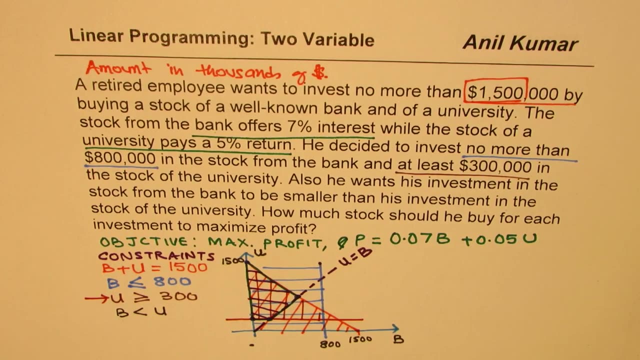 so. so that forms the solution space for us, correct? so we're looking into this area now. now, clearly, the two points which we should be testing are these two points which will give us some clue of what should be our solution right now. remember, this is a dotted line. it's kind of 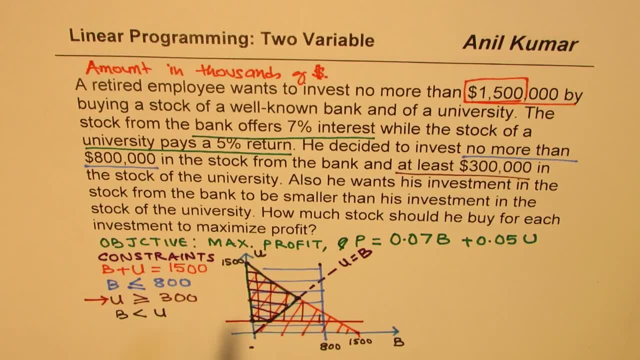 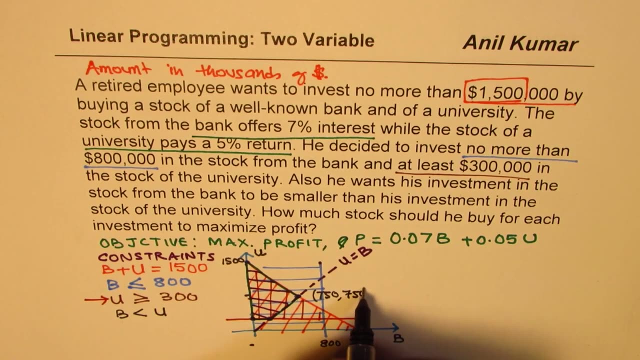 slightly different. we don't have greater than equal to so. so this point of intersection basically, is 750- 70. so we're going to have a point here. we're going to have a point here, we're going to have a point: 0, 1, 0. we can see that right at the end we have an equivalent of 450, right? so 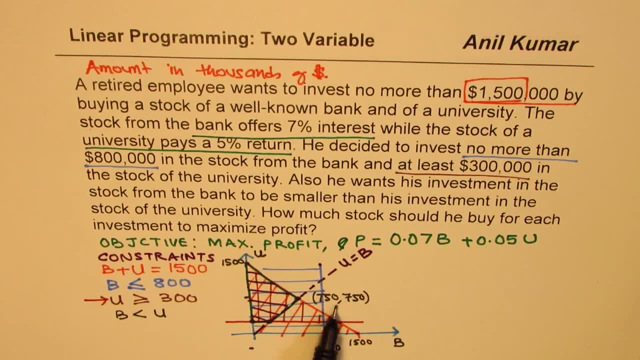 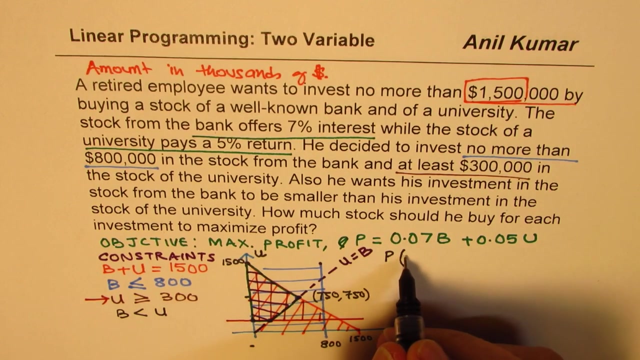 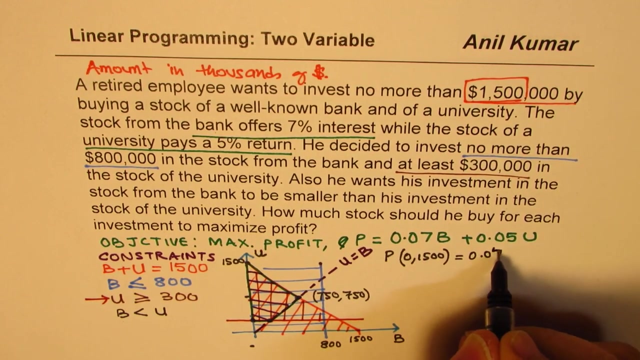 it is right. so what we need to do is to check the profitability from these two points right and see what do we get. so if I use all as university being x very, very safe, then this point is zero for bank. so the probability when we use uh 0 and 1500 will be 0.07. sorry, 0.05. 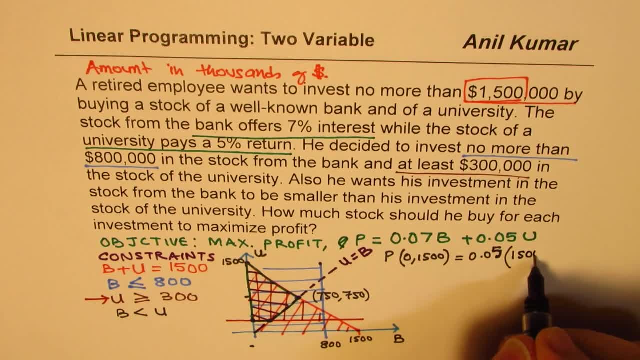 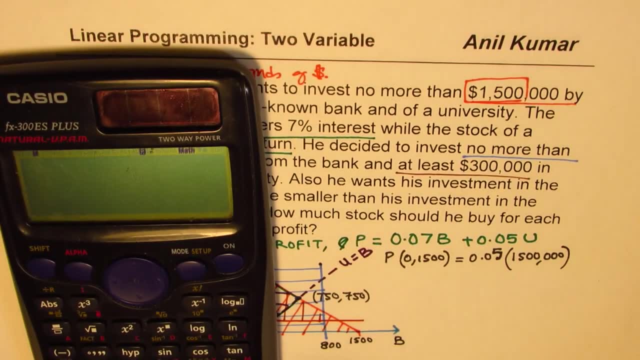 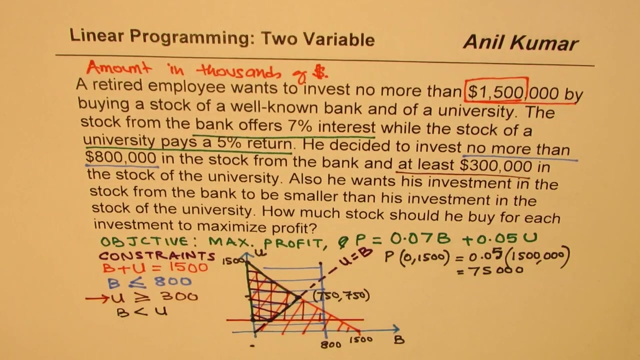 times 1500- and remember this is per thousands. we'll add thousand here. so that gives us the total profitability. so, which is 0.05 times 1500, 000 and that is equal to 75 000. okay, and if i use this, i cannot use this actually, right, since this is on the line and we want. 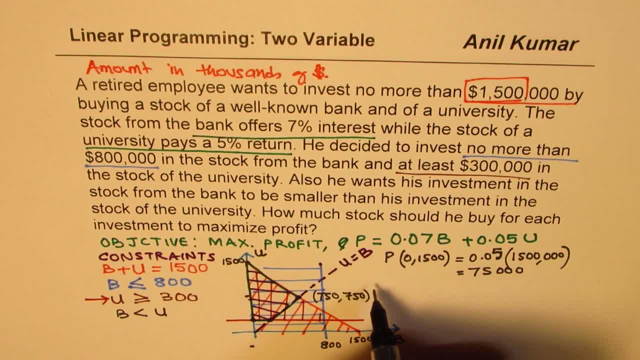 the university to be higher. so what we could do here is that we can actually use a point where it is 749 and 751. so we can use 749 and 751, correct? so let's use this. so it is 0.07 times 749 000 plus 0.05 times 751 thousand. 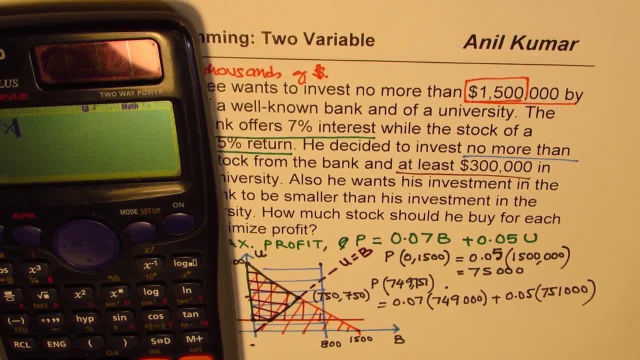 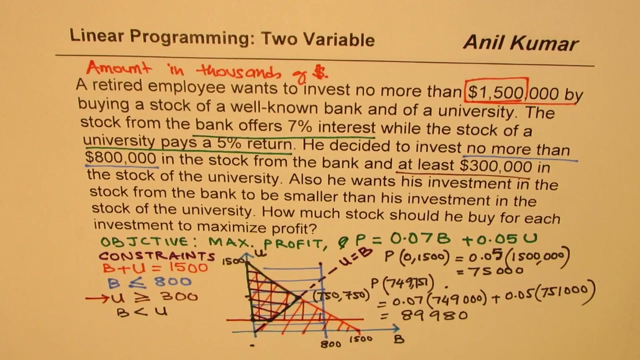 so we get 0.07 times 749 000 plus 0.05 times 751 thousand and that gives us 89 980, 20 short of 90 000. so that is the amount, and clearly this is much higher, and therefore our suggestion is, from this situation, that in the university, 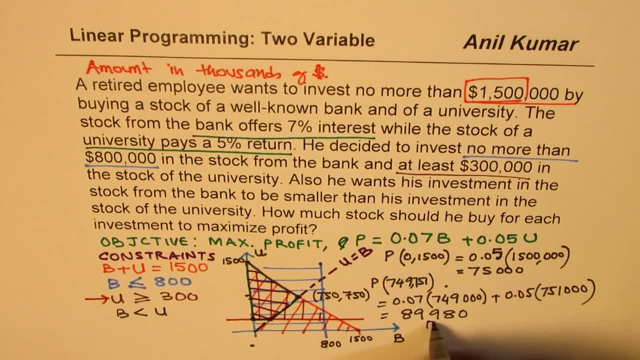 and the bank. the distribution could be so: for the bank it is 749 and for the university it is 751, so that will satisfy all our conditions. so we have invested more in the university than in the bank, university paying slightly lesser returns- five percent- as compared to that of the bank, of seven.